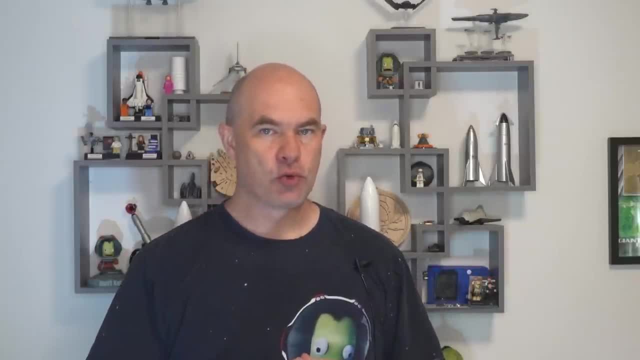 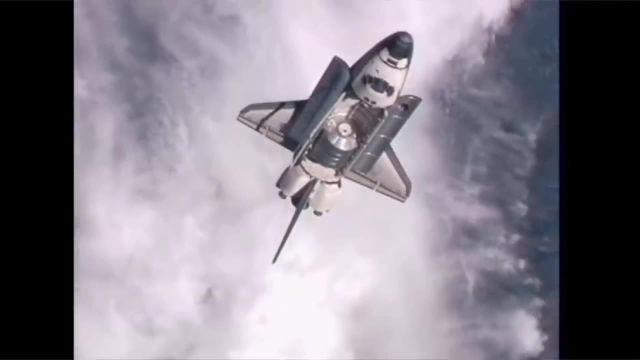 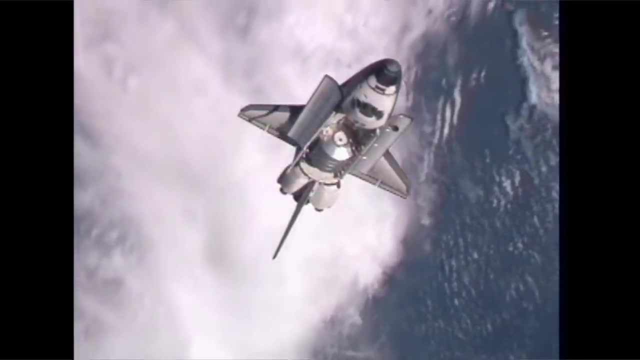 the moon. The space shuttle was designed to ferry crew and payload only to low Earth orbit, And while it was a very capable vehicle for operations in low Earth orbit, it was limited in the maximum altitude it could achieve. I believe the highest altitude a shuttle ever achieved was just over 600 kilometers. 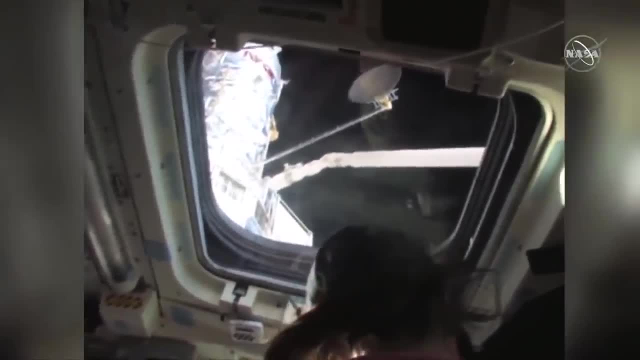 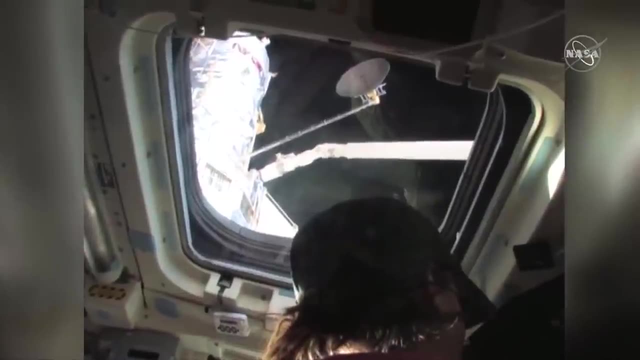 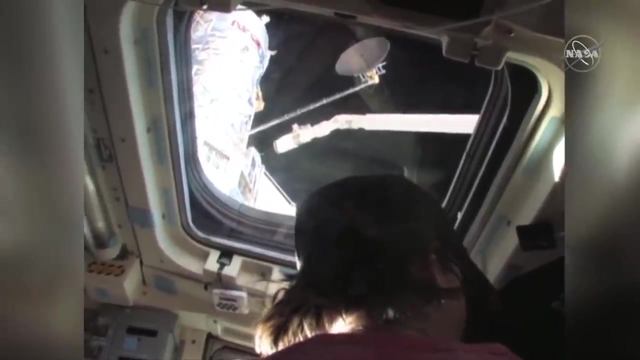 when deploying and servicing the Hubble Space Telescope. But it was possible for a shuttle to go higher than this. It was just a trade-off with payload versus propellant. However, it's not clear just how much higher it could go, since there are a lot of variables involved. So the standard shuttle 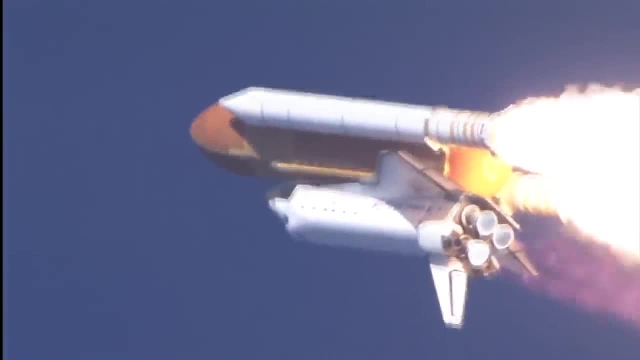 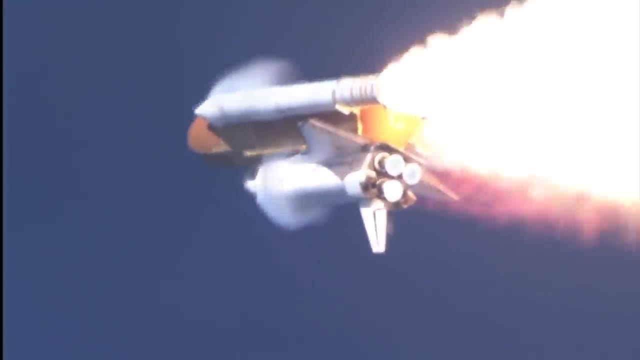 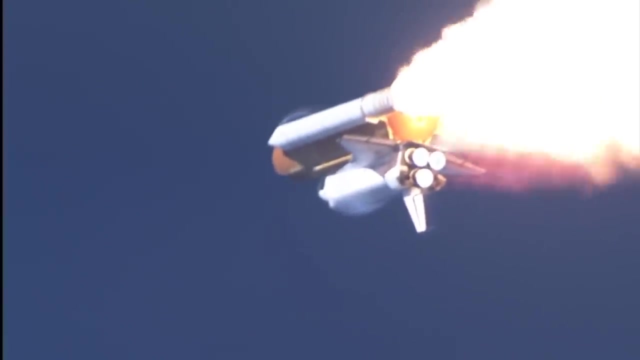 would fly to orbit using the solid rocket boosters and the three RS-25 main engines, which run on hydrogen and oxygen that's taken from the external propellant tank. The initial target orbit would be elliptical, with a perigee of around 60 kilometers, so that the external tank would re-enter quickly. 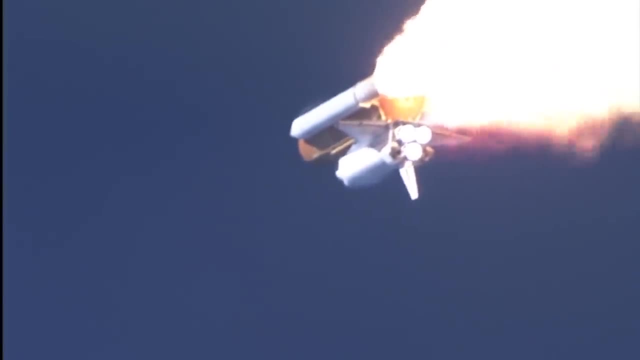 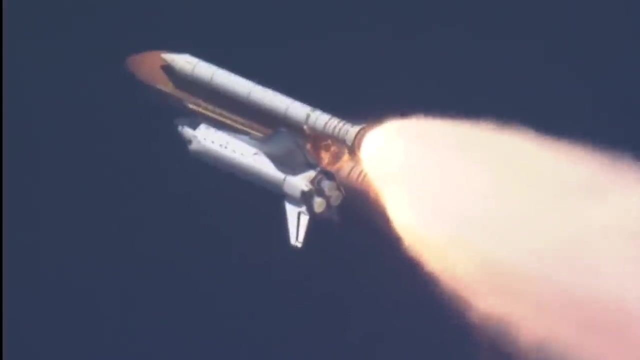 after being jettisoned To keep the orbiter in orbit, the shuttle needed to make a second maneuver in orbit, but it couldn't use the powerful main engines because they didn't have any propellant. Instead, the shuttle would switch over to using the orbital maneuvering system. This was a 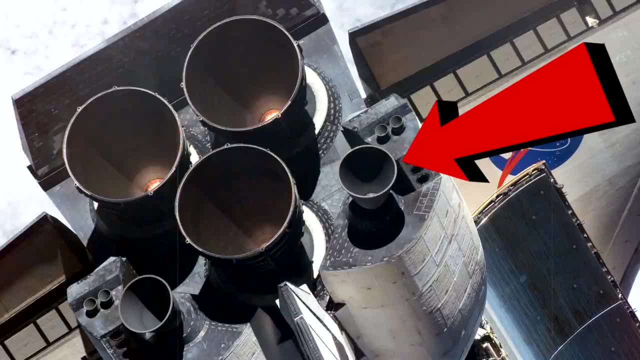 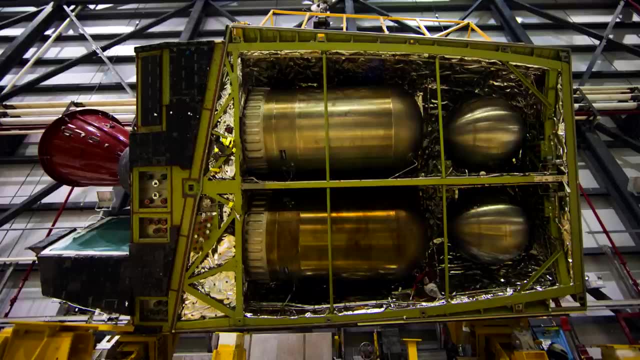 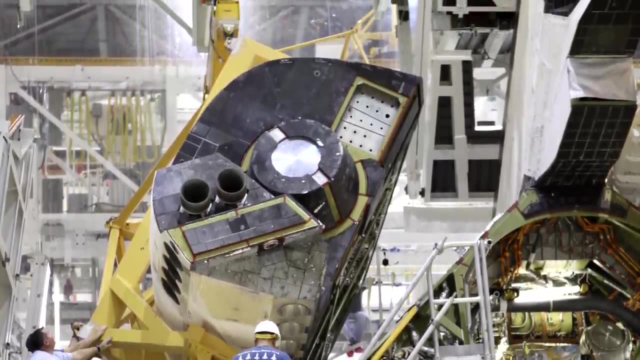 pair of AJ-10 engines running on hypergolic nitrogen tetroxide and monomethylhydrazine. The orbital maneuvering system could carry up to 13.5 tons of propellant and had about 300 meters per second of delta-v, which is pretty respectable. The shuttle was quite a capable vehicle, while in 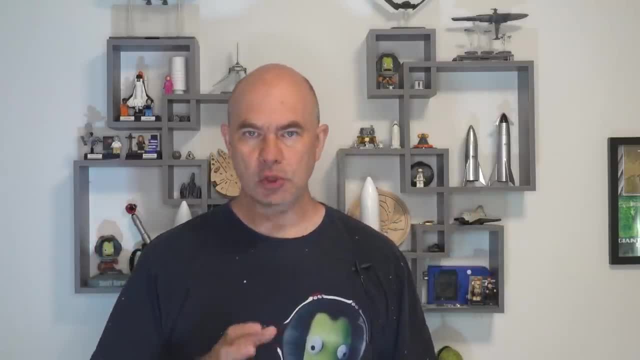 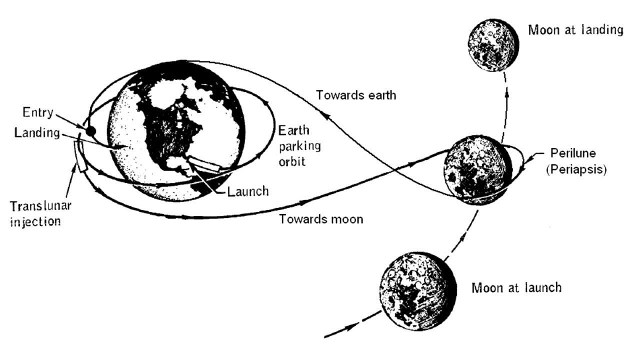 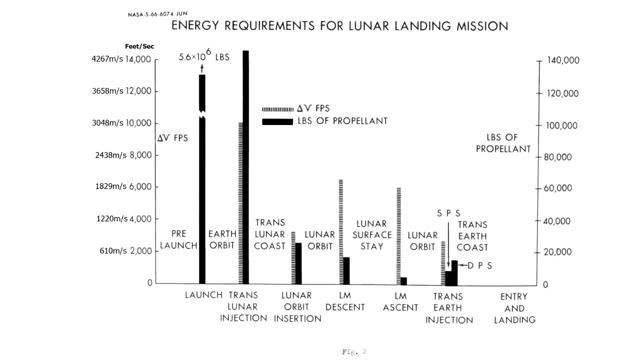 orbit. So what does the shuttle need? to get from low earth orbit to the moon and then possibly into low lunar orbit and then maybe, hopefully, back to earth? Well, starting from a 200 kilometer orbit and boosting into a transfer orbit that flies out to the moon. that needs about 3-3.1 kilometers. 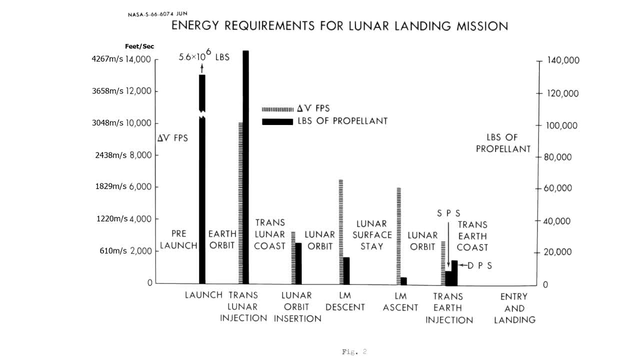 per second, depending upon where the moon is. But then that will just fly past the moon unless it can slow down there To capture into a lucid, bound eccentric orbit- that's probably another 200 meters per second- And to get into a low lunar. orbit. from that that's another 600. So from there, of course, if it then wants to get back to earth, it will need the 600 and the 200, so that's another 800 meters per second from low lunar orbit. to get home, So from low earth orbit, the shuttle in the trailer would have needed at least 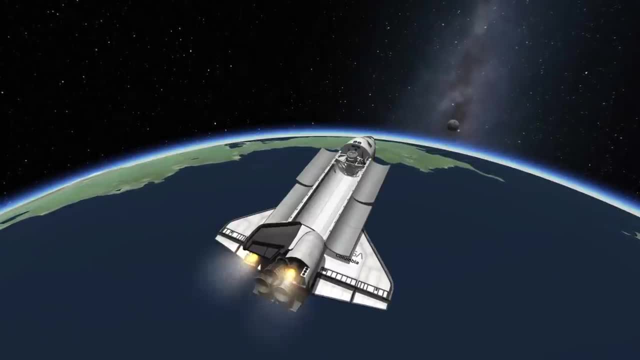 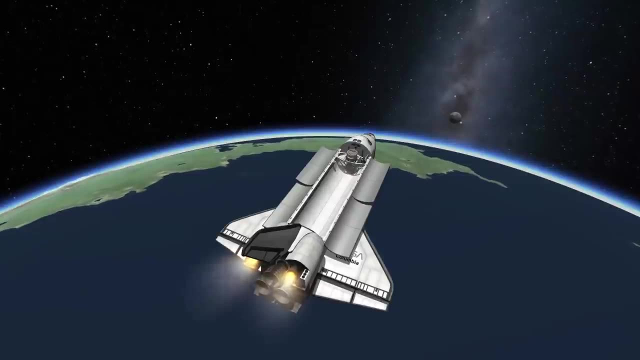 3.1 kilometers per second for a flyby and probably as much as 4.7 for lunar orbit orbit in return. So clearly the orbital maneuvering system needs more propellant beyond what it's designed for, And the good news is that the designers of the shuttle had anticipated that. 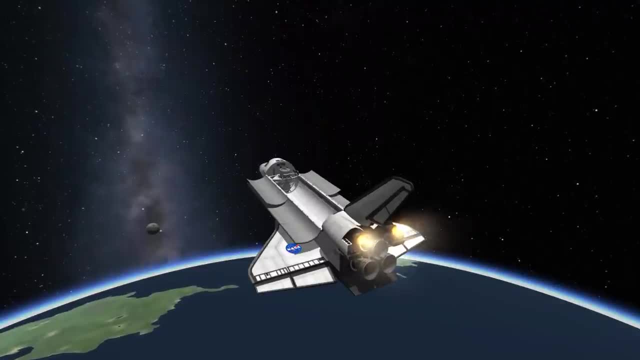 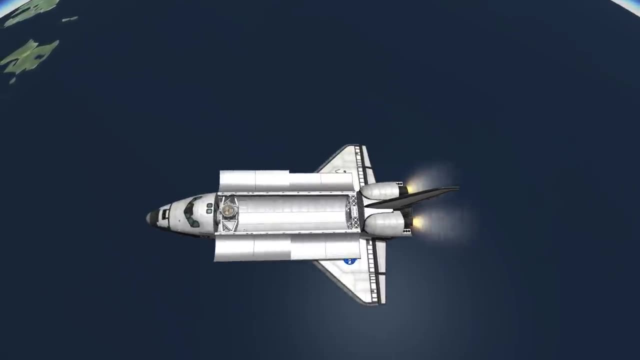 there might be missions where they needed more propellant than could fit in the tanks. So there was a concept of the OMS payload bay kit, which would carry extra propellant reserves inside the payload bay And the shuttles all had the plumbing to hook up these tanks and controls in the cockpit. 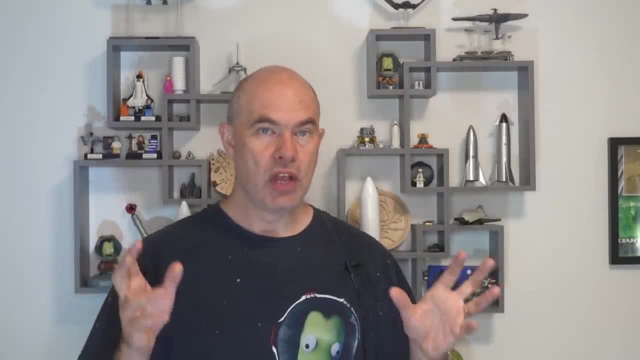 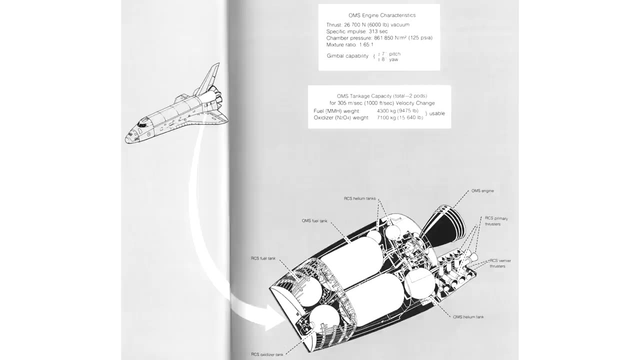 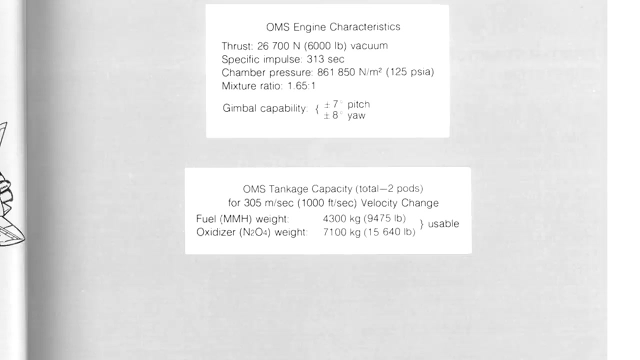 for them. It was never used, however. So how much extra propellant would we need? Well, NASA documents tell us that the AJ-10-190 engines would get a specific impulse of 313 seconds, and the rocket equation says that we need 175% of the shuttle's dry mass in propellant to reach the 3.1 kilometers. 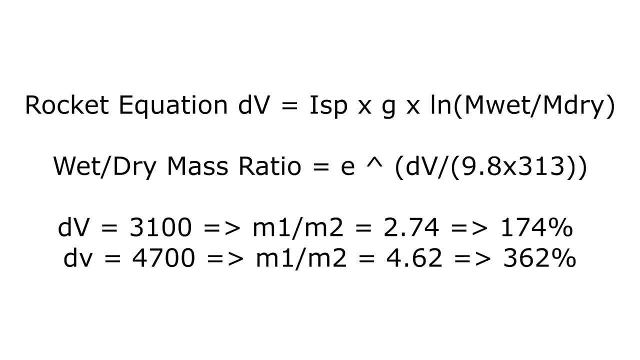 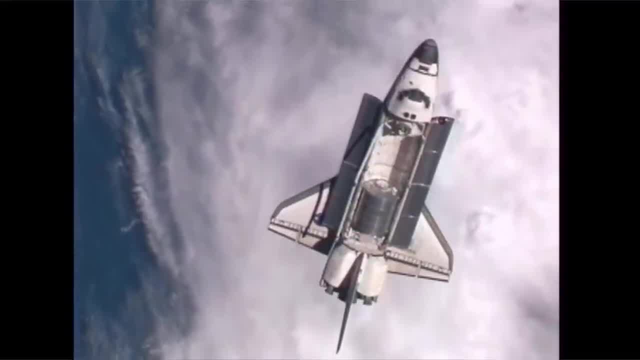 per second and 360% of its dry mass for an actual low lunar orbit. So for the dry mass of the shuttle let's just assume 80 tons. But in truth that's with no payload and not much in the way of other. 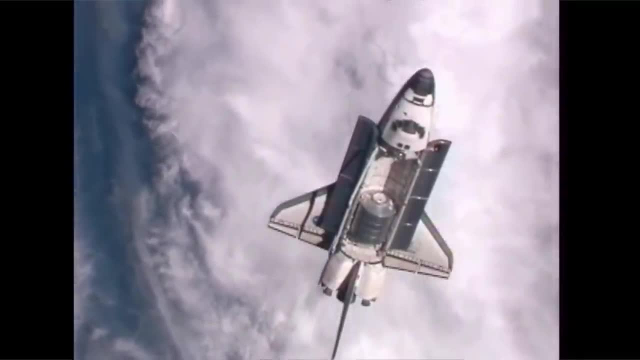 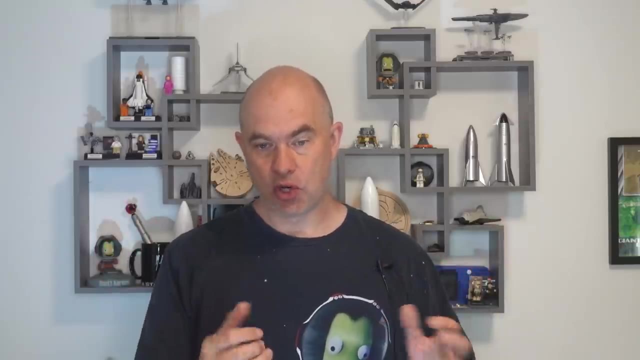 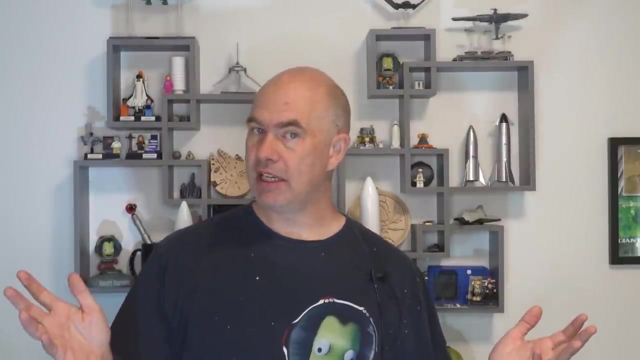 consumables. But that gives us fuel requirements of 140 tons and 290 tons. The density of monomethyl hydrazine and nitrogen tetroxide in the correct mixture ratio for this is about 1.2 tons per cubic meter. So can we fit that in the payload bay? Well, the shuttle's payload bay is 300 cubic meters. 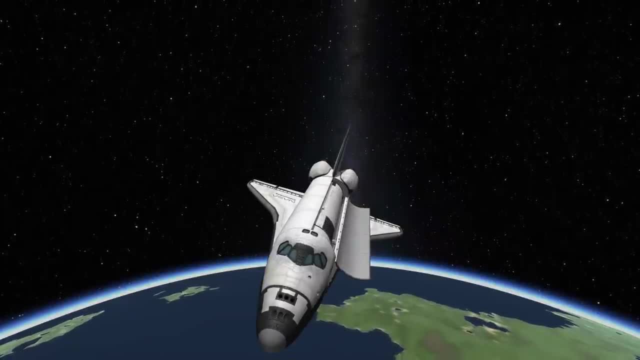 That's based on the shuttle's payload bay, So we can fit that in the payload bay, So we can fit that in the cylinder. 60 feet long and 15 feet wide. That's a nice and roomy and while it would be a bit of a. 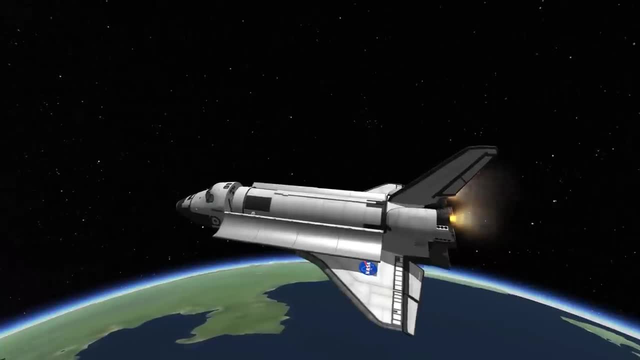 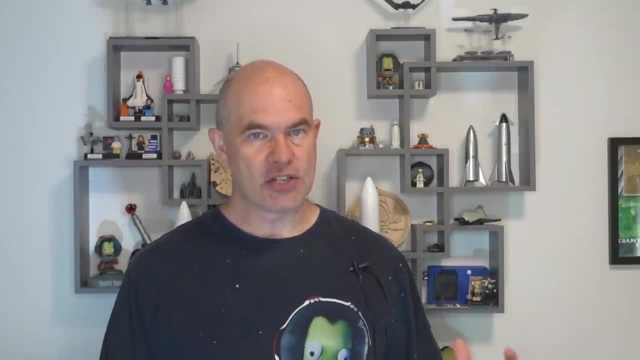 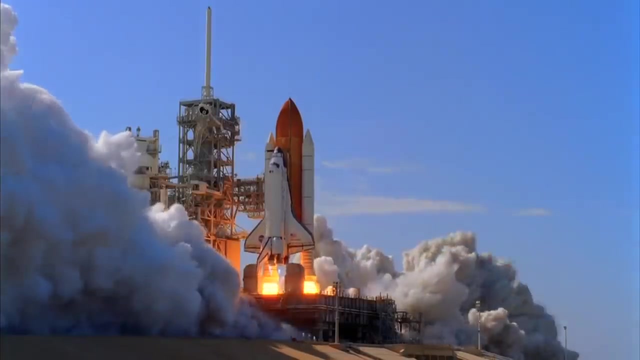 squeeze, it would just about accommodate the propellant for both Delta V requirements, which all sounds very neat, but it would never work. First up, it would never get into orbit. The payload capacity of the shuttle was more like 25 tons, so you're never going to get it. all the 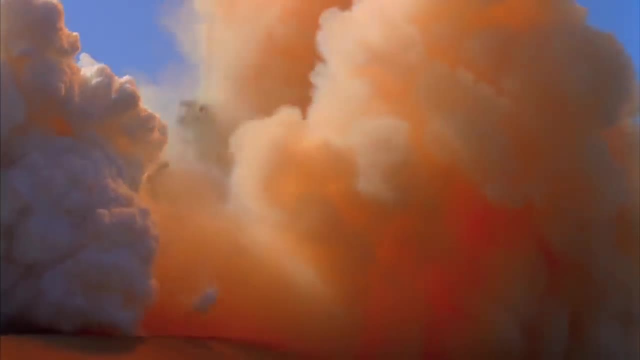 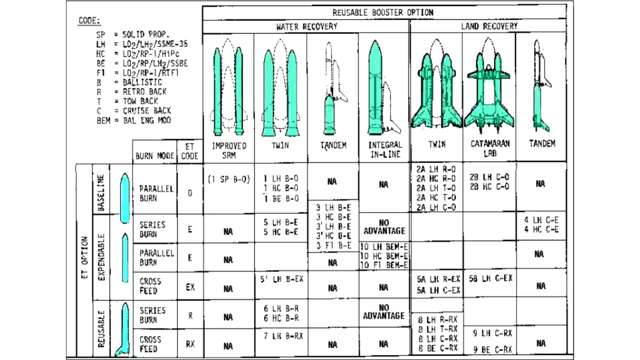 way up into orbit if you add hundreds of tons of ohms propellant to the payload bay. Now, granted, there were shuttle concepts that raised the payload mass by changing the launch system, adding boosters, but in the trailer we see a regular space shuttle configuration. 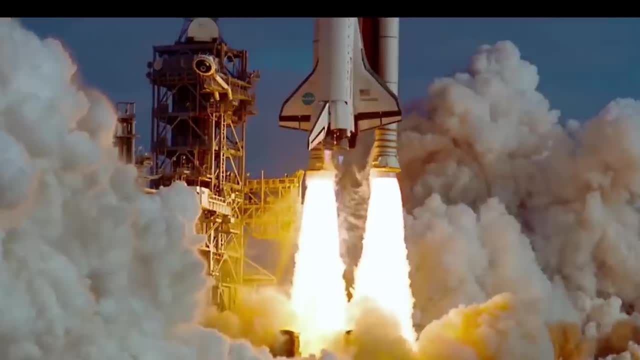 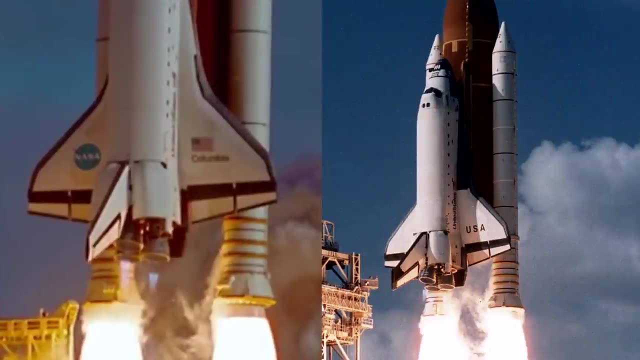 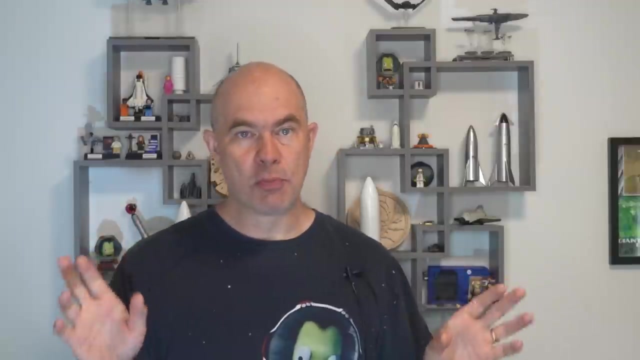 launching. I might also mention in the trailer the black and white tile patterns on this version of Columbia don't match the real one. In fact it looks like the leading wing edge of the elevons don't match between the two shots in the trailer. Look, the point is we can rule out some super. shuttle upgrade that would make it to the moon. Secondly, the ohms thrust was really low, so that acceleration to escape velocity or lunar escape would take far too long. They would either have to waste Delta V due to gravity losses or they would have to do it in multiple passes. 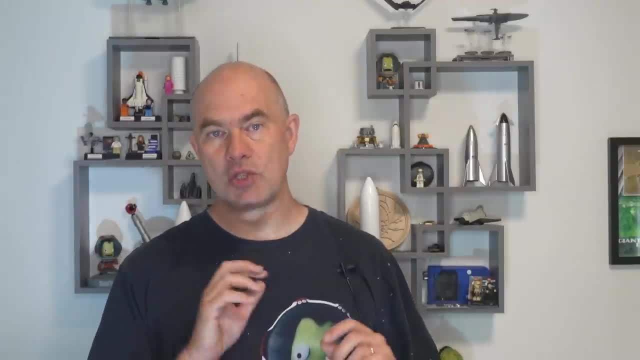 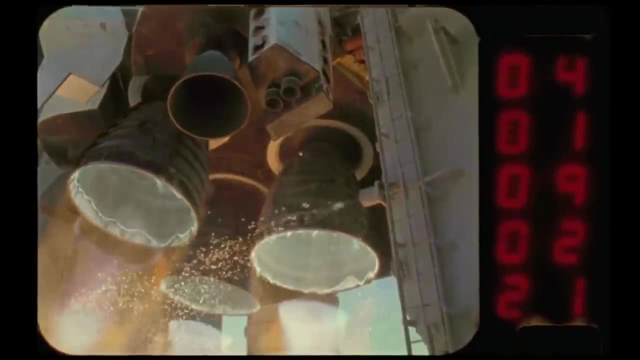 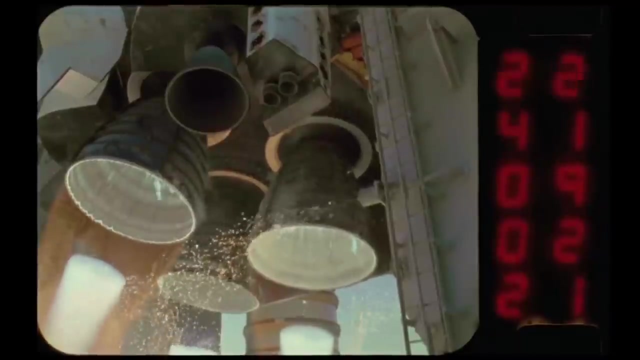 and that would mean many, many passes through the Van Allen belts, which is not good for your crew. So there are the main engines, which are much higher thrust and much more efficient. How about we fill the payload bay with hydrogen and oxygen tanks? Well, Hydrolox is about one quarter. 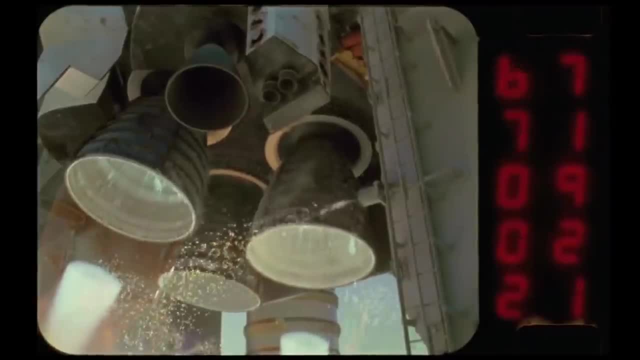 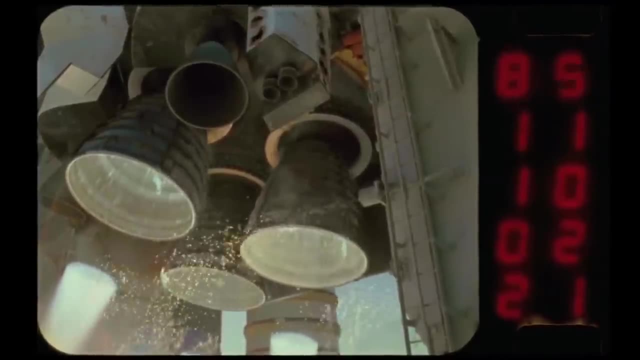 the density of the hypergolic fuels. so you're only going to fit about 84 tons into the payload bay, which gives us about three kilometers per second of Delta V barely getting to fly past the moon with a bit of the help from the ohms thrusters And, of course, if you fill the entire payload bay. 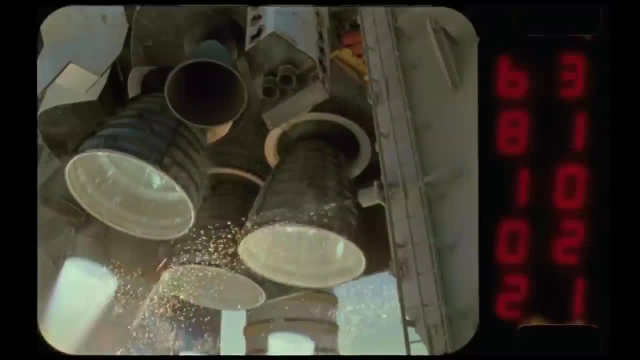 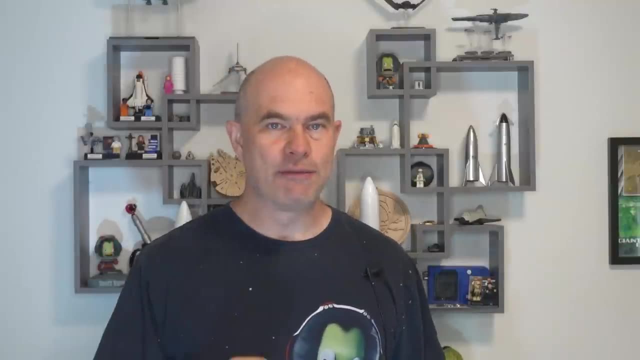 there's no room for payload to take to the moon, which kind of makes the whole thing pointless. So I'm sorry for doing all that math because there's a better solution and one that makes far more sense in the- you know- environment of the TV show. I think that they have to refuel in 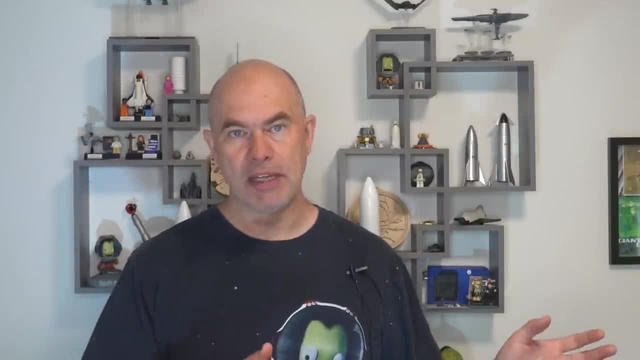 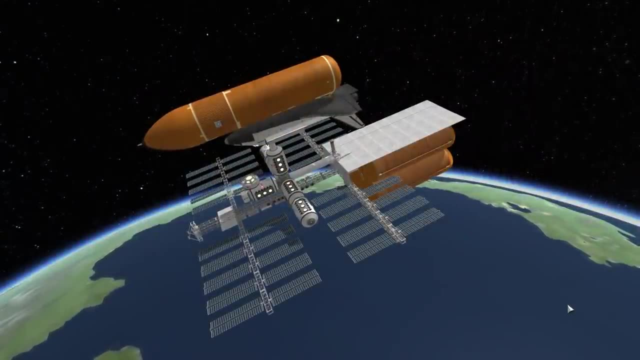 low Earth orbit, and instead of refueling the ohms and filling up the payload bay, they'd simply keep that large external tank and refuel the hydrogen and oxygen at the space station. The show talks a lot about water on the moon as a resource, so maybe they harvest it from. 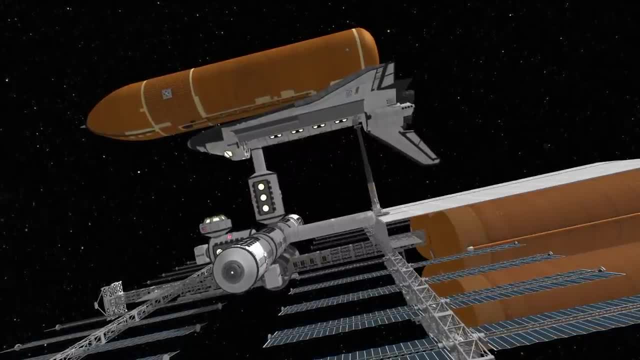 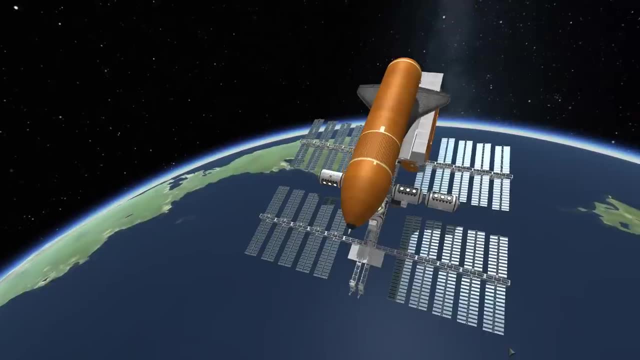 the moon and bring it down to low Earth orbit. Or maybe they just have fuel ferries that are bringing up propellant from the surface of the Earth. If your show is built around having a large base on the moon, having a station in low Earth orbit is well within their technological capabilities. 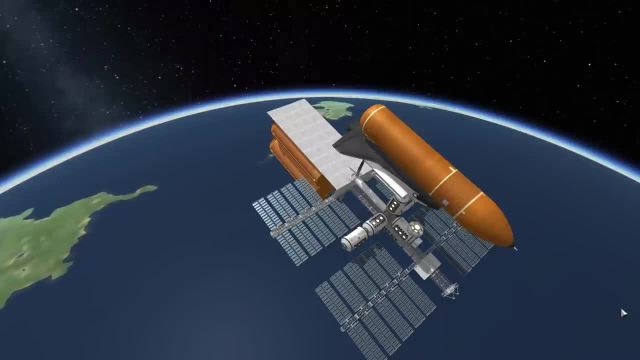 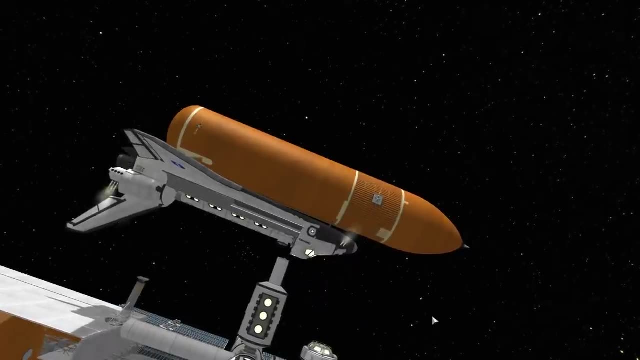 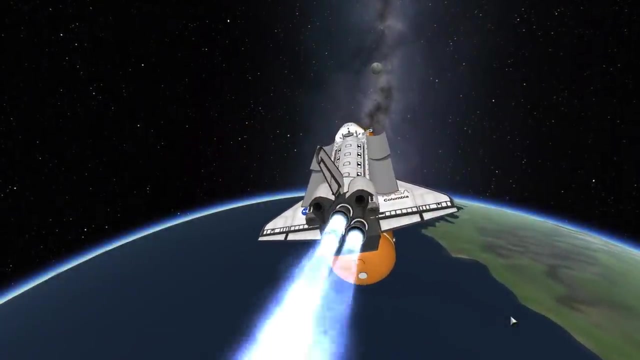 So, anyway, the external tank does add a bit of dry mass, but the huge volume would let them put enough propellant in there to perform the entire lunar injection, orbit, insertion and departure, and it would leave room in the payload bay. I wouldn't try landing it though, because those wings are just dead weight on the moon. 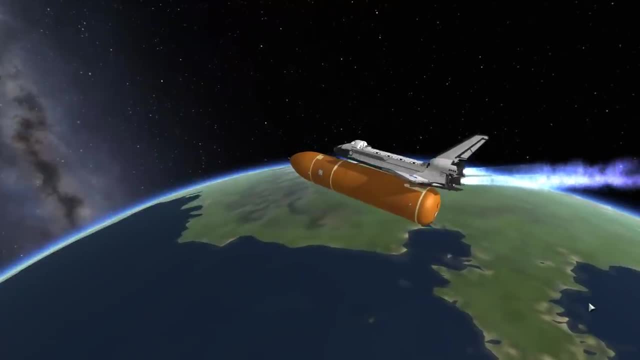 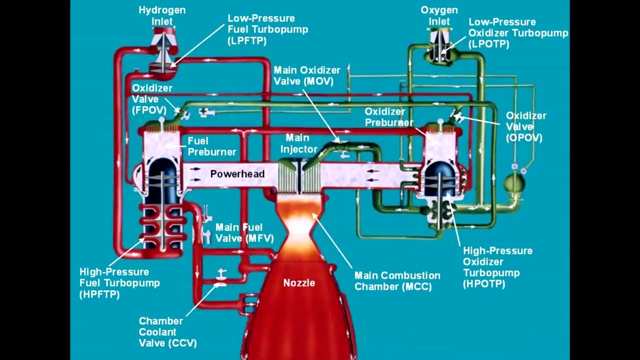 The RS-25 engines were never started in flight at any point, but they were designed to need nothing more than pressure of the propellant and electrical power to start up. So, in combination with a knowledge burn from the ohms thrusters, there's no real reason that they couldn't be. 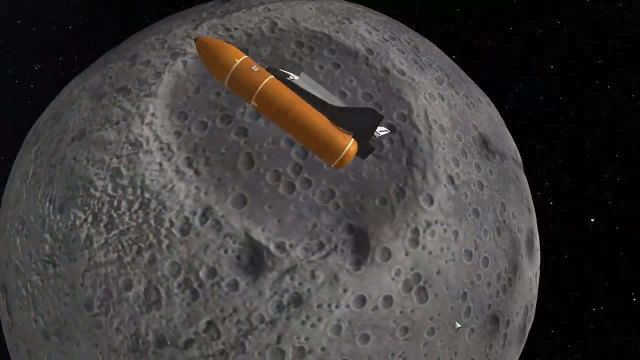 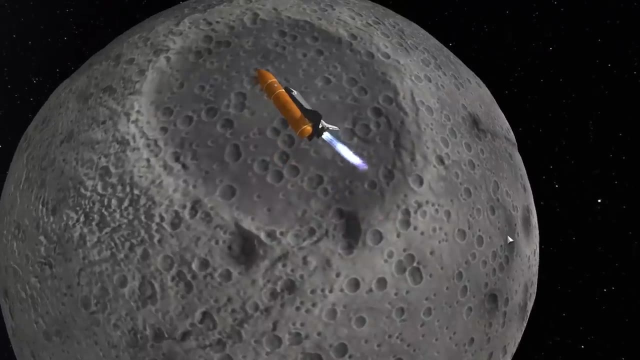 used multiple times in flight. The other technical limitation would probably be the evaporation of the liquid hydrogen over a multi-day mission, But the tank has capacity for over 700 tonnes of propellant, so I'm sure they would just load extra propellant and deal with it. 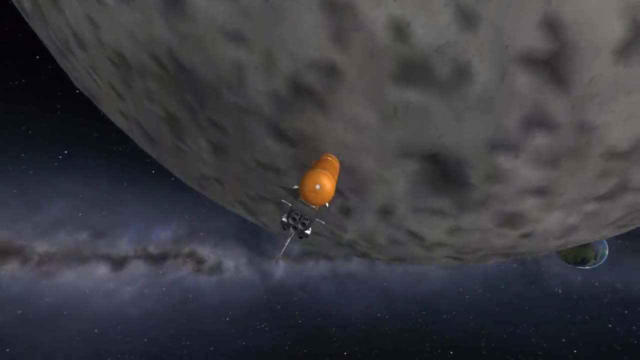 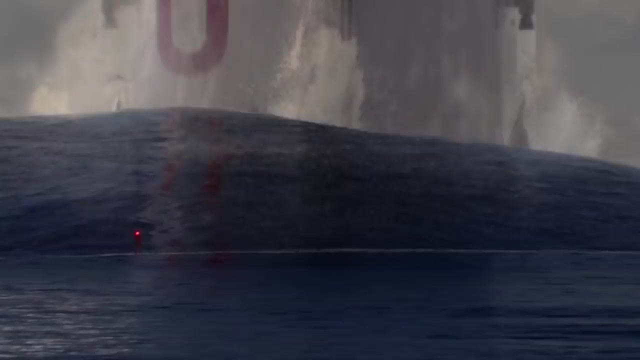 Now the other option for the TV show might be some kind of space tug. They have a post-credit sequence in season one that puts a nuclear-powered spacecraft on top of a sea dragon, which honestly seems a bit out of place in the evolution of Apollo to the shuttle. but maybe they want to have a. 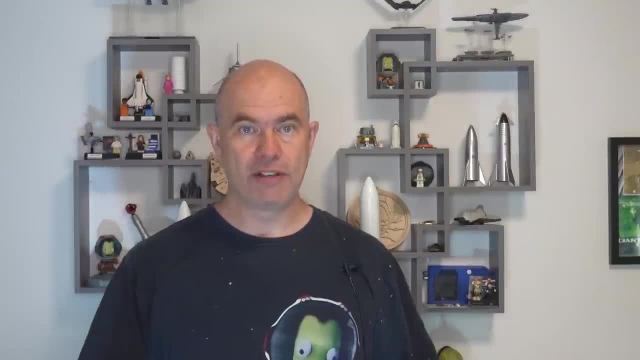 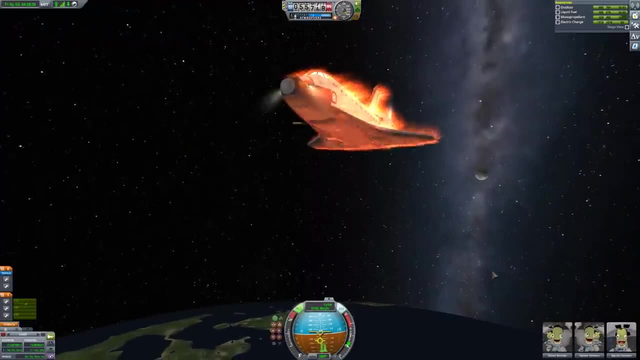 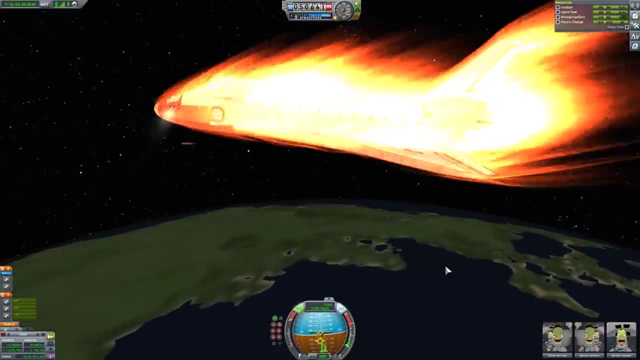 space shuttle and bring it to the moon Either way. there's one final problem that affects both possible solutions: The thermal protection system on the shuttle would not be able to handle return from lunar orbit. The total heat load is more than double and the peak heating higher still. 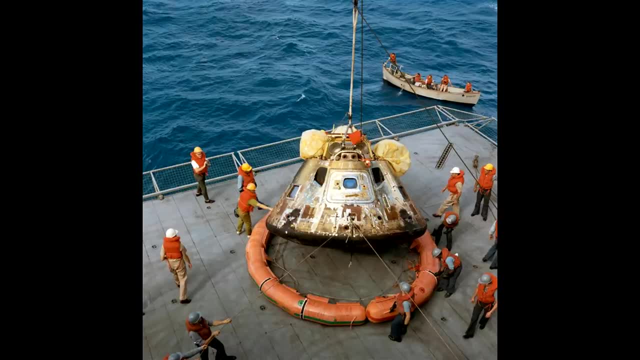 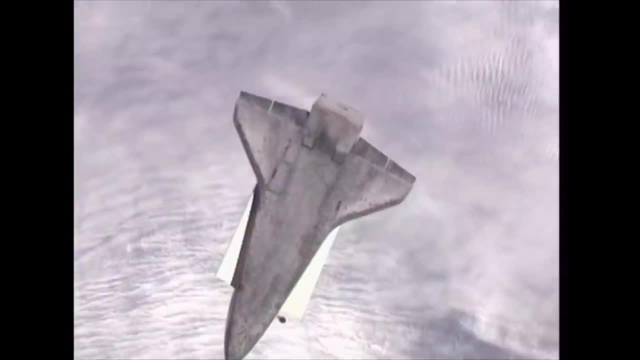 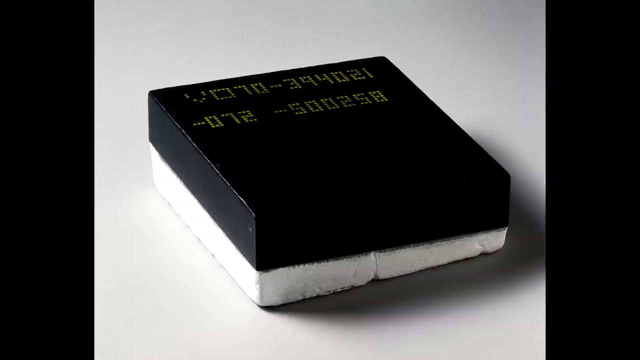 compared to low Earth orbit. Apollo had a single-use ablative heat shield, but the shuttle had to be reusable And, as designed, those thermal protection tiles would need to be a lot thicker to protect the shuttle from a lunar re-entry. The top of the shuttle might be better off being silver. 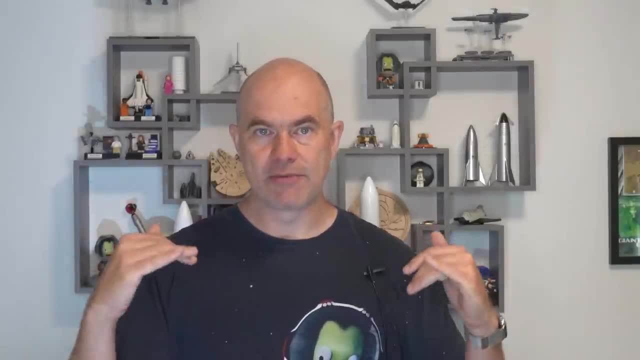 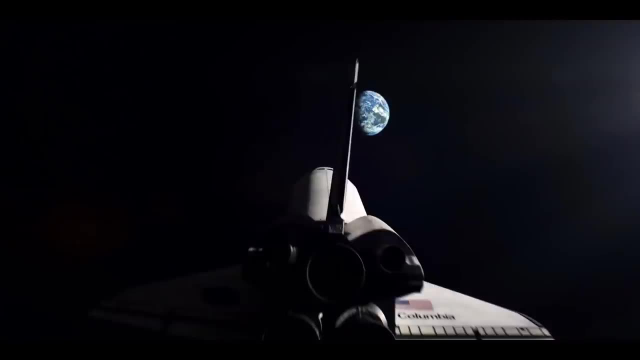 as well to reject more of the radiative heat from the plasma trail. Finally, it's worth commenting that the shuttle is shown headed back to Earth and has its payload bay closed, And this is probably a mistake, since the shuttle's thermal control system needs the doors open to expose the 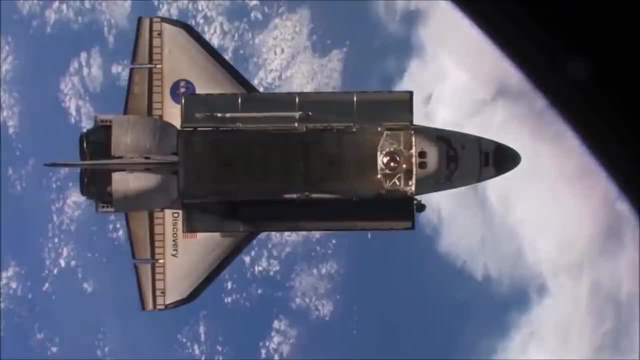 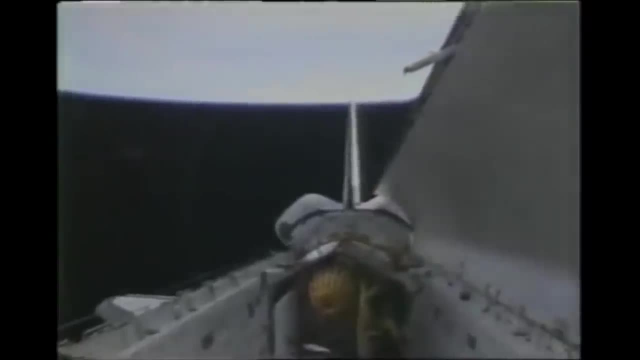 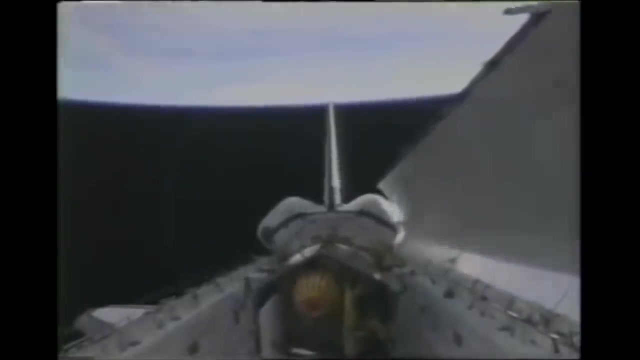 radiators. However, this system is designed to operate in low Earth orbit, where the heat flux is higher, as the Earth reflects and re-radiates energy onto the spacecraft. The thermal management in deep space may well be a little different, but I still think the doors should be open. 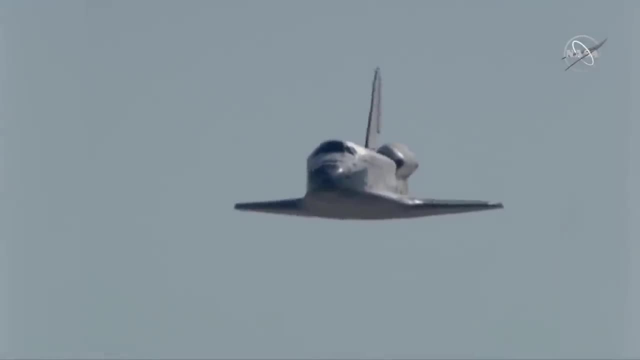 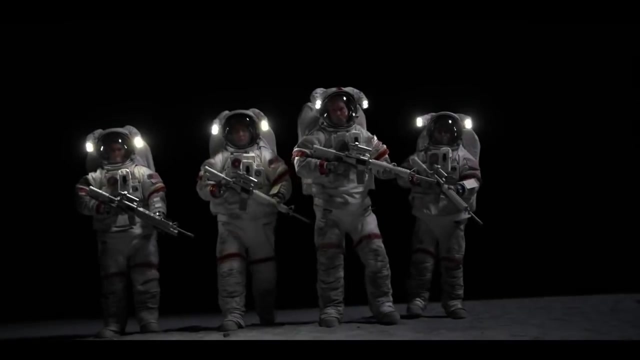 Anyway, taking the space shuttle to the moon is generally a bad idea because the shuttle has so much extra mass for systems that aren't useful at the moon, things like wings. But hey, it's just a TV show and it's set in an alternate history and it's clearly interested in